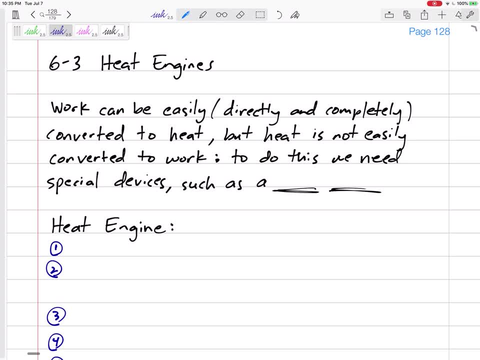 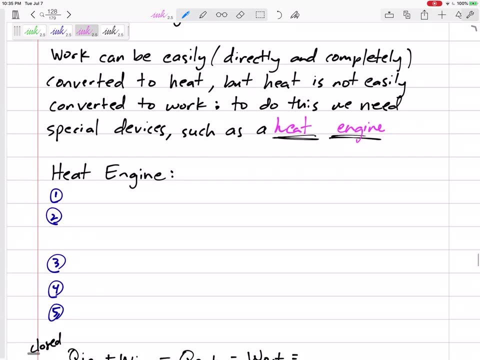 to spin the paddle wheel right. It doesn't go backwards quite as easily. In order to convert heat to work, we need a special device like a, A heat engine that we'll talk about. A heat engine. Okay, a heat engine. 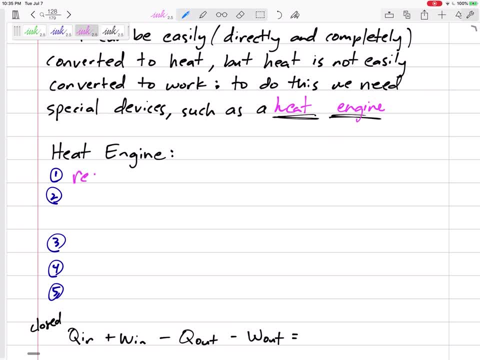 it receives heat, receives heat from a high temperature source, All right, then it converts that heat or part of that heat. it converts part of heat to some work, to some work out, some work done by our system, Usually by a, Usually via a rotating shaft. 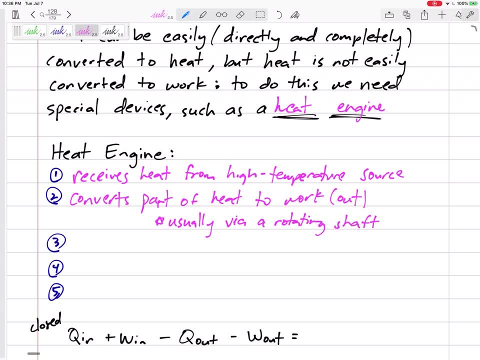 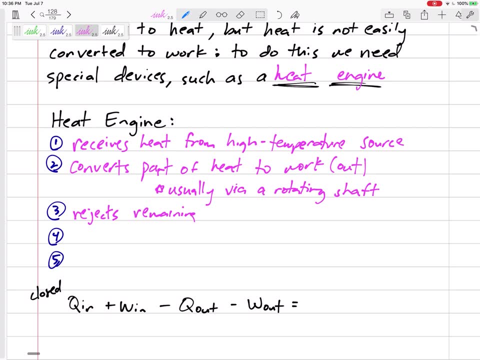 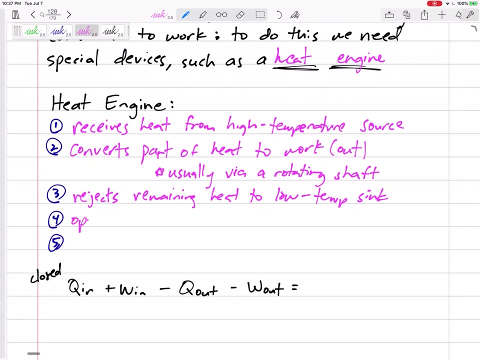 And then it rejects The remaining heat To a low temperature sink. To a low temperature sink. It operates on a cycle. So whatever states and whatever properties it started with, after it gets the heat converts to work, rejects the heat, it comes back to its starting conditions, operates on a cycle and it usually 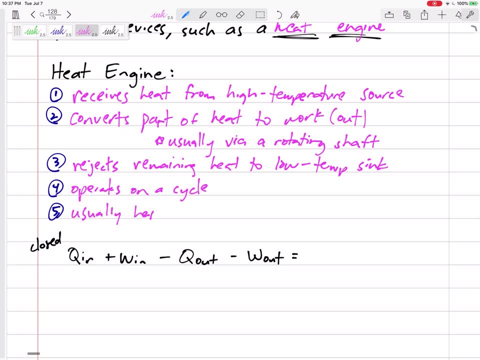 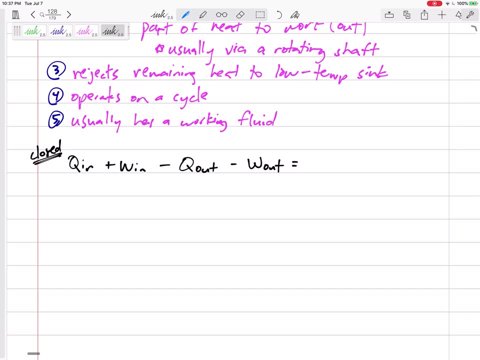 has a working fluid, usually has a working fluid, refrigerant water, air. usually it has a working fluid, alright, and usually it's a closed system, or we can we think about it as a closed system, alright? so if it's a closed system, then Q in and W in minus. 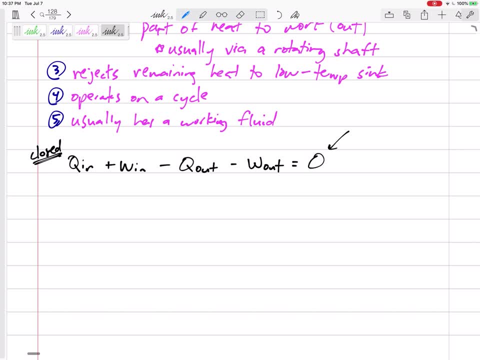 the Q out and W out equals zero if it's on a cycle right, if there's no change from initial, you know, and then one hour later to final, if it comes back to its original energies. our conservation of energy equation is this right here? so maybe we'll put the 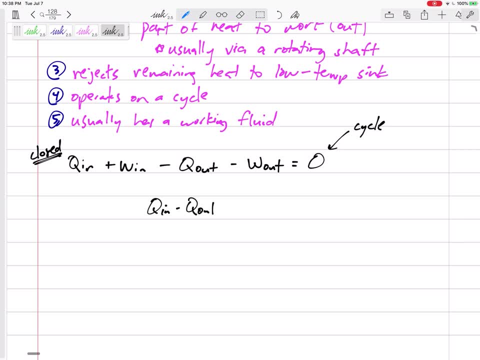 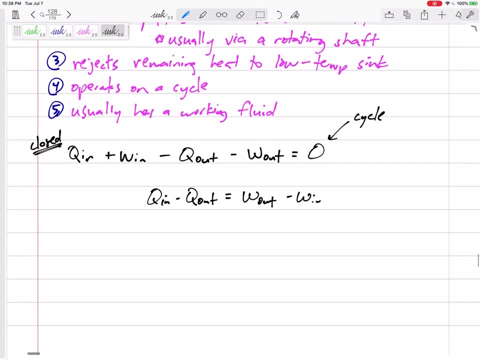 Q's on one side, Q in minus the Q out. alright. so if it's a closed system, then Q in minus Q out. let's put the W's on the other side, the work out minus the work in. so let's say: 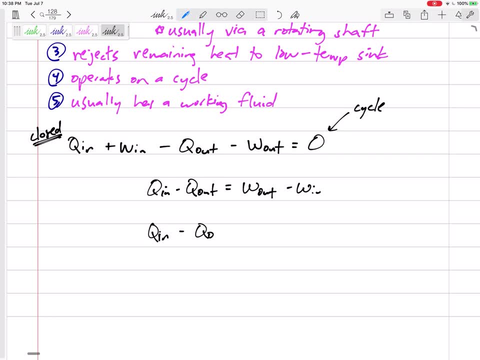 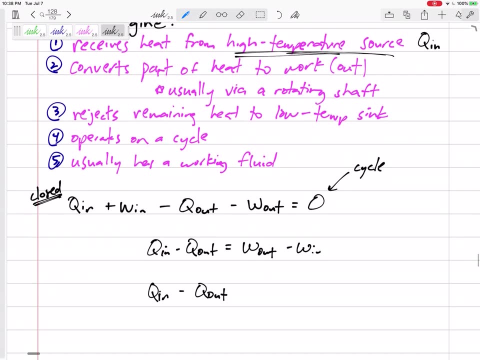 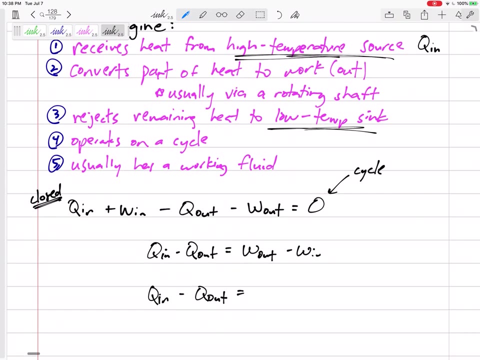 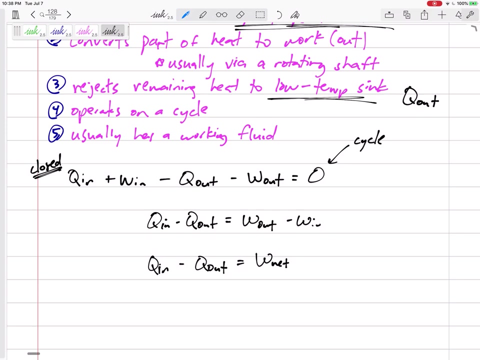 the Q in that it gets from the high temperature source. right, this is Q in minus the Q out. so it rejects to the low temperature sink Q out. Equals: work out minus, work in. so the work net right, work net. 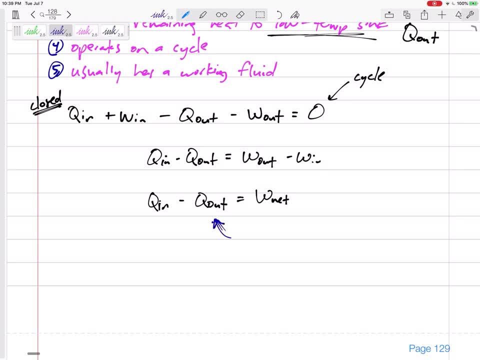 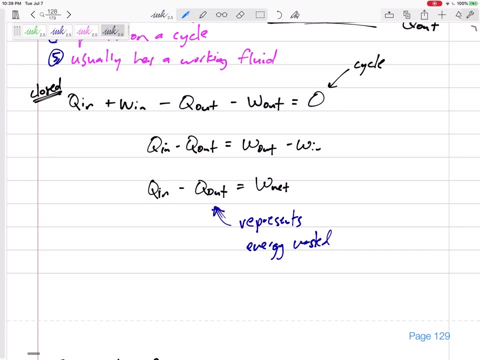 This Q out represents the energy wasted. Q out represents energy that is wasted, And we're always going to have some energy wasted, So we end up having to put in more Q in than the net work that we get, because some of that Q out is wasted. 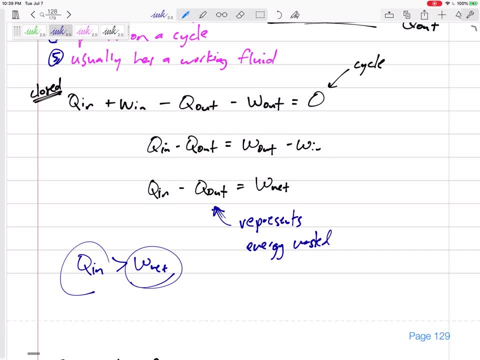 But hey, at least we do get some work. you know, maybe we are putting in a lot of Q, we're putting in a lot of heat, but we are getting some work out. You know, we are rotating, we're taking heat, I don't know- fire, spark ignition. 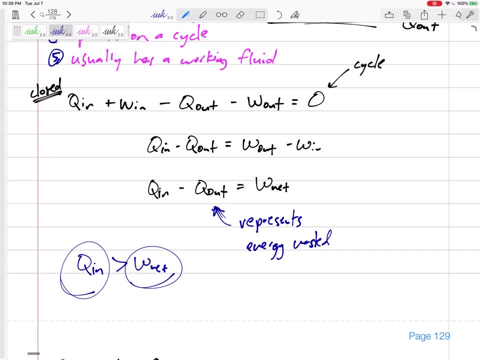 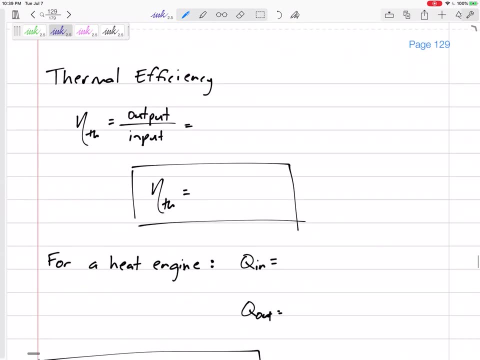 and we are maybe pushing something, rotating something and getting some work out from that heat. Okay, thermal efficiency, and this is of heat engines- thermal efficiency of heat engines is this: eta subscript TH: thermal eta, eta subscript TH Efficiency is output over input. 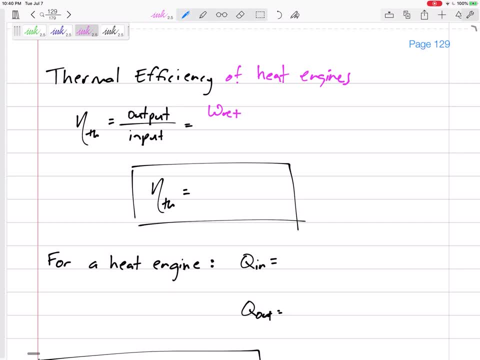 What is the output? What are we getting? We are getting out work, net. okay, The work, the net amount of work is what we're interested in. That's the work. that's the output. What are we having to put into it? 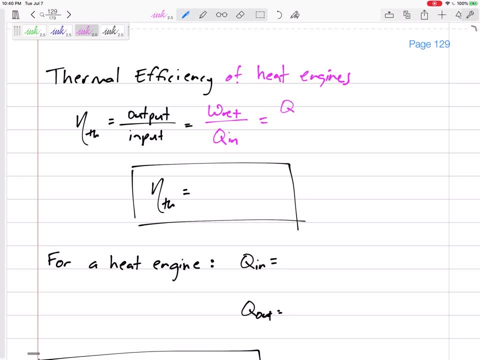 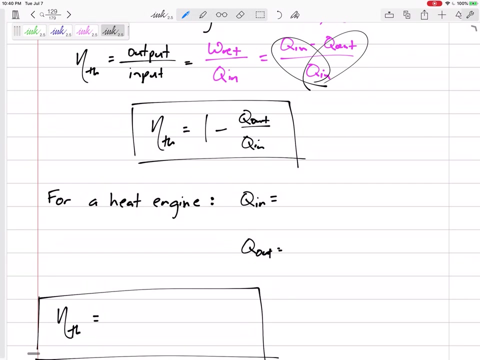 Q in. Or I know that work net is Q in minus Q out over Q in. Let's just subtract both of those. This is one. let me write this one right one: minus Q out over Q in. Alright, For a heat engine, the Q in is the Q from the high temperature source. 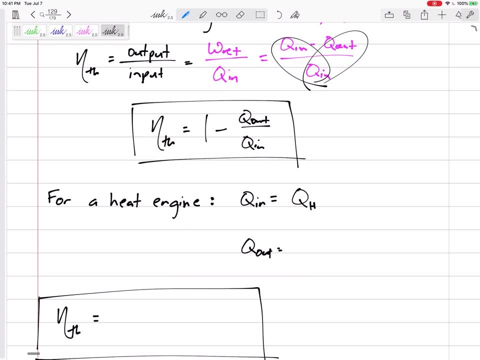 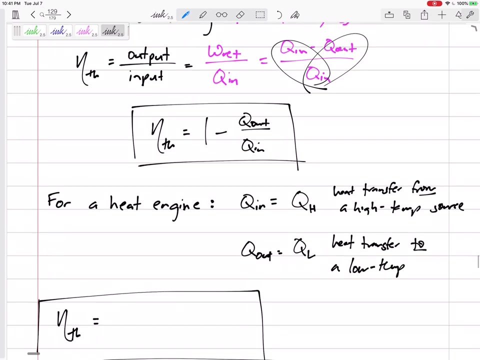 So I'm going to say Q- hot or QH. So this Q in is QH, We're going to call it. this is the heat transfer from a high temperature source, Q out is QL, Q- low temperature. And this is the heat transfer to a low temperature sink. 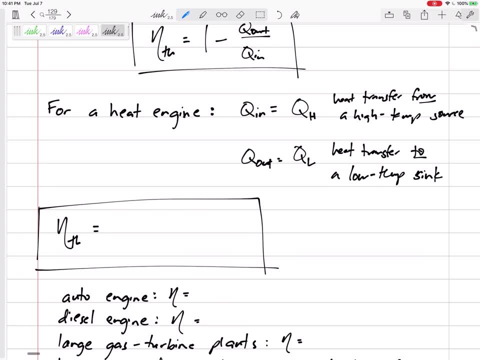 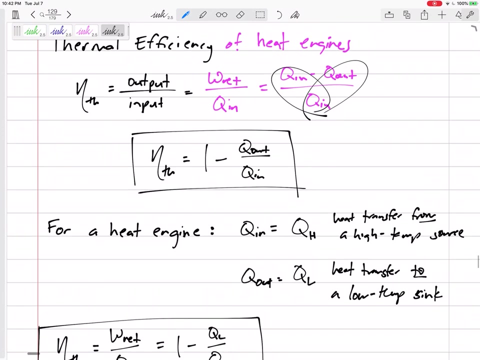 So eta is work net over QH or one minus QL over QH. So a lot of different formulas that we've got here So we've got to kind of juggle these around. Work net is QL, QH minus QL, right. 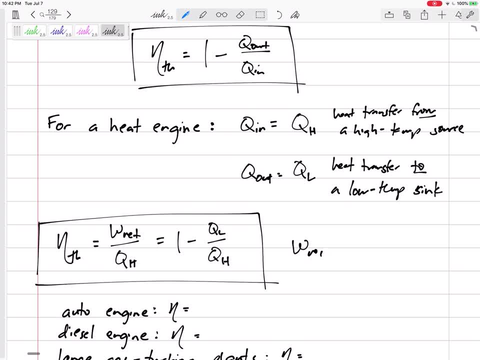 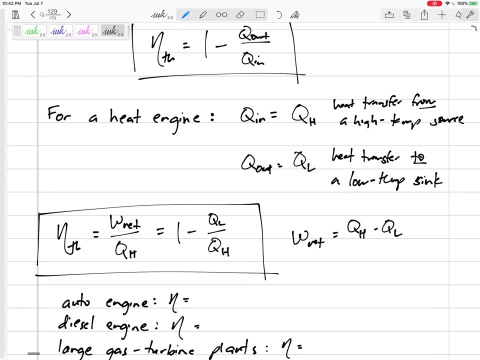 And here's another one: Work net is what Q, let's see Q in Q, H minus QL. eta is work net over QH. also one minus QL over QH. Okay so, and let me go to the link. 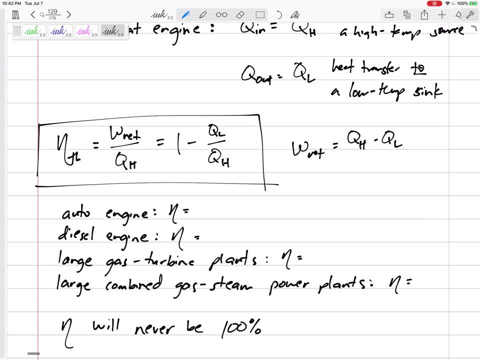 I hope that I'll send you a link of animation of a four-cylinder, I think, engine. It's pretty cool to look at. But what efficiencies are we looking at? How much heat do we convert to work? For most car engines, eta is. 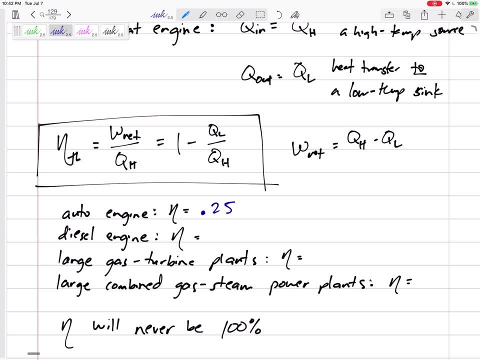 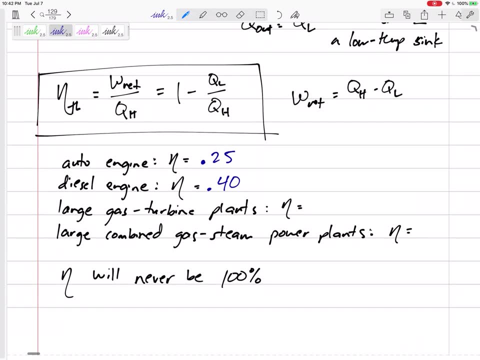